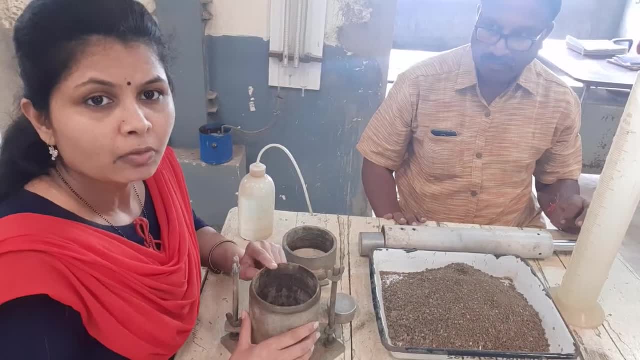 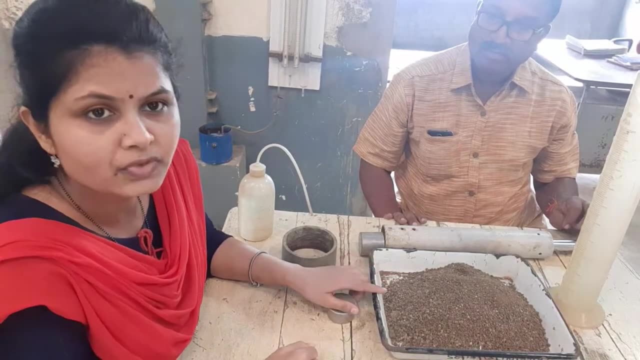 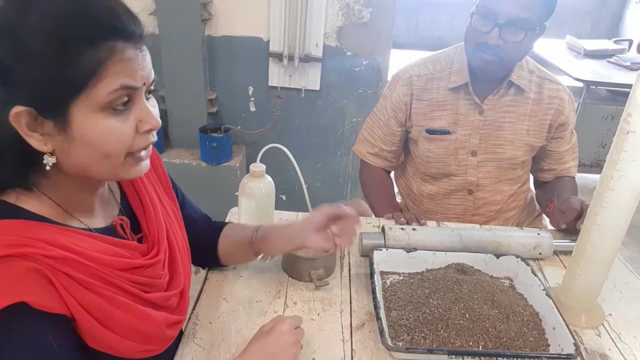 We have to not attach this collar. We have to take the empty weight of this mould. The next step we have to perform is we have to take 2 kgs of sample, that is, ISC, from 4.75 mm sieve. Then we have to add the water percentage wise. 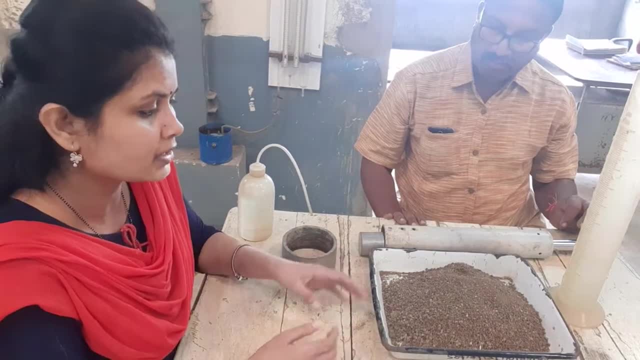 So we have to take. we can take any kind of percentage, like, for example, I am taking 15% of water is to be added for 1 kg of soil, But we are having 2 kgs of water, But we are having 2 kgs of water. 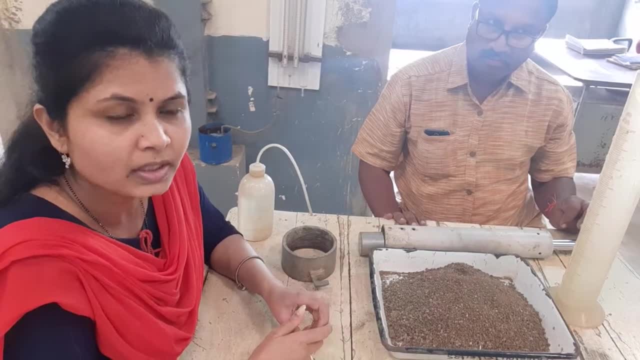 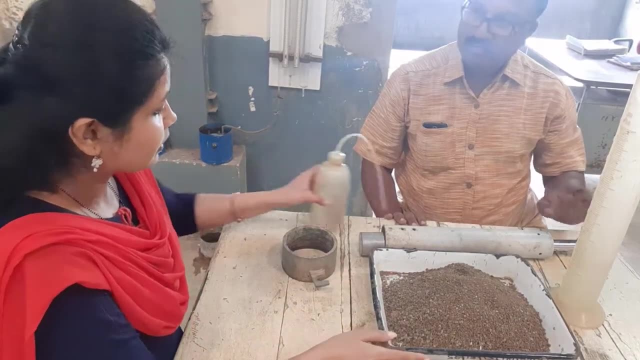 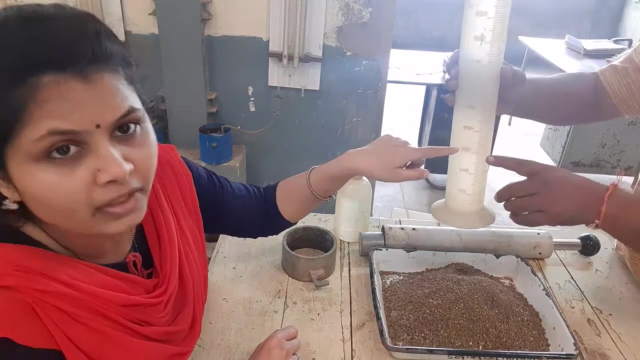 So 15 will become double, that will be 30%. that means 300 ml of water we have to add to this soil, So we will first measure the soil into the measuring jar. so we will require a big measuring jar. It consists of a 300 ml of water. 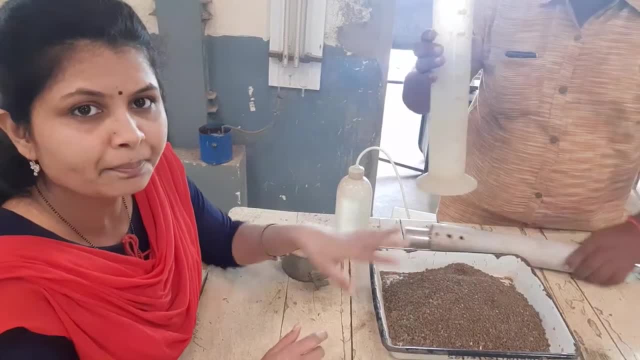 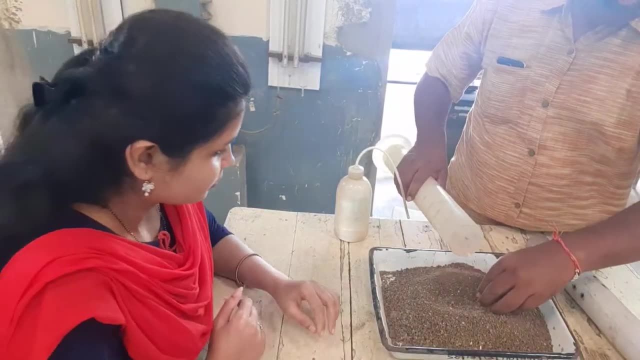 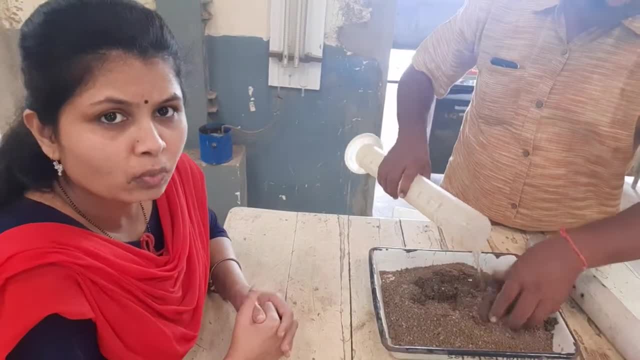 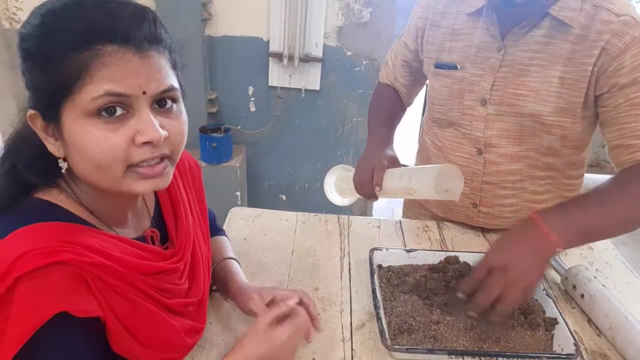 Then we add the water temperature which we have. slowly, We will gradually add on water. We will add the water slowly, slowly, step by steps, and we will mix all the soil so that it gets moist, all the grains of the soil gets moist. 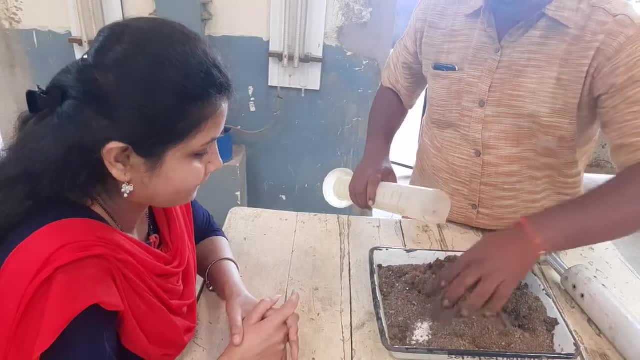 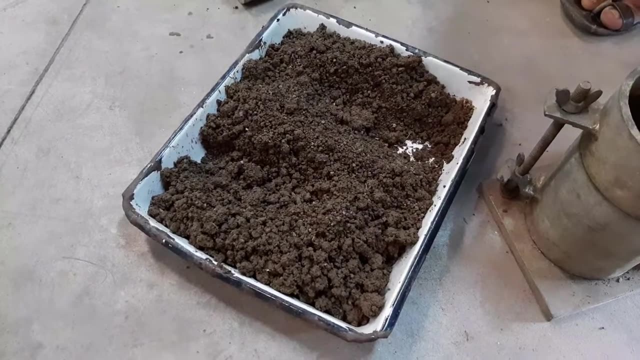 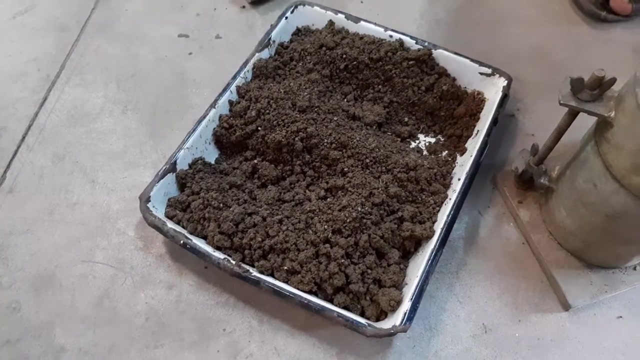 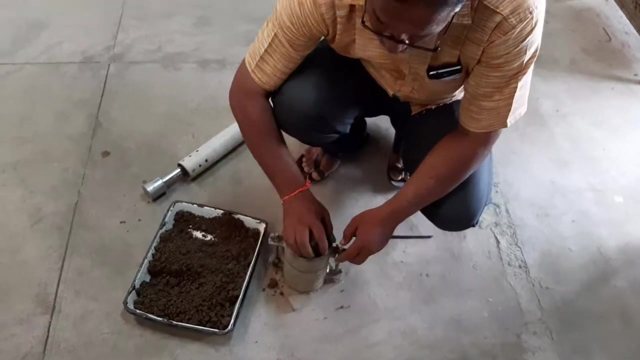 Now, after making the paste or adding the water to the soil, we have to make the make: 3 parts of the soil sample that we have collected in our tray and part wise we will fill the soil into our compactor mold. we'll take the first part of the soil and we will add to the 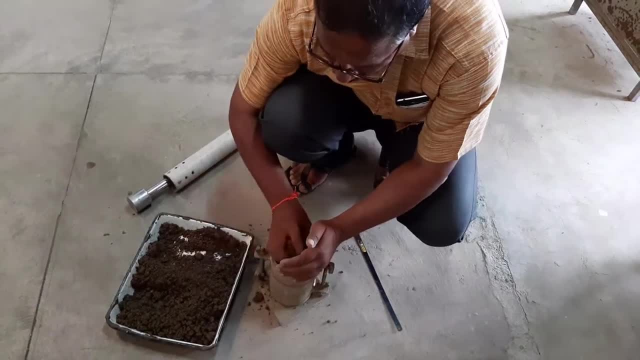 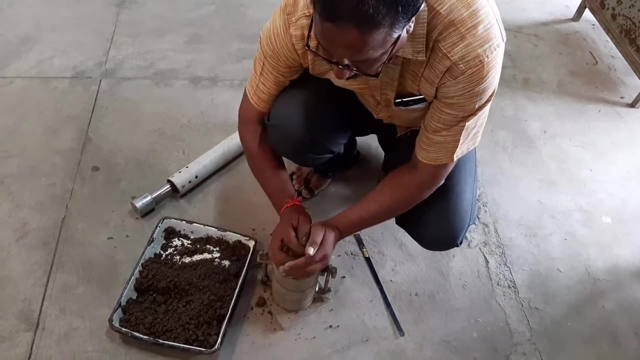 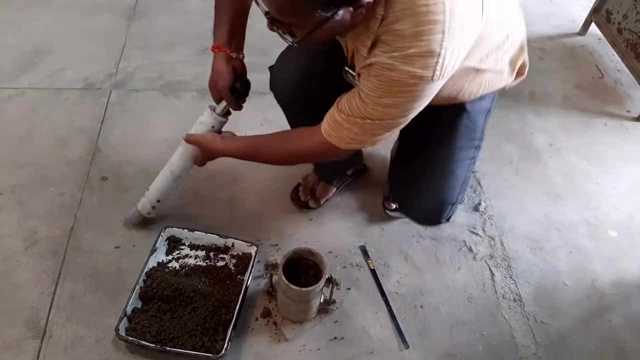 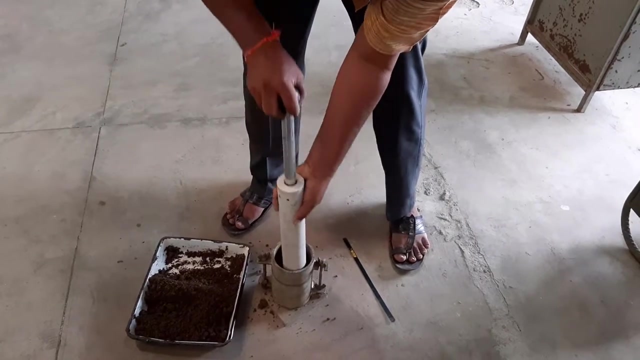 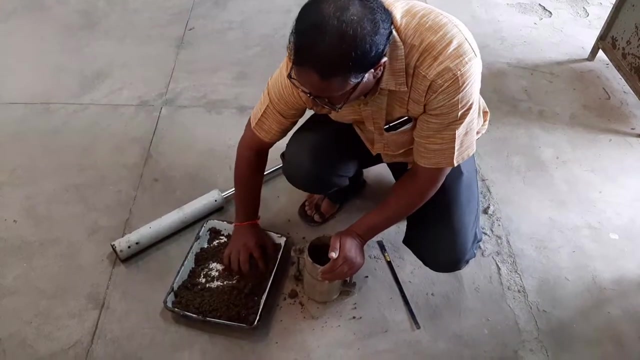 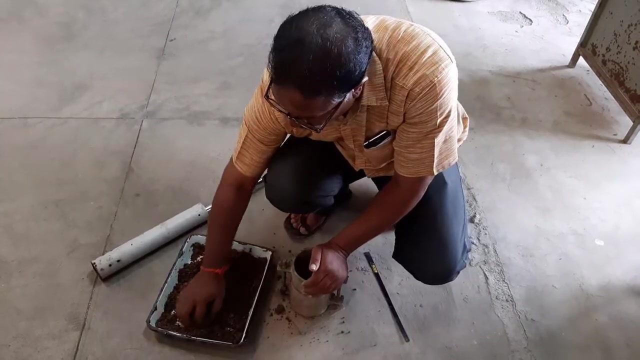 compactor. after filling up the first part of the soil, then we will use the steel rammer and we'll blow 25 standard number of blows to compact the soil. then we will add another set or another part of the soil to the compactor and then we will again use the steel rammer. 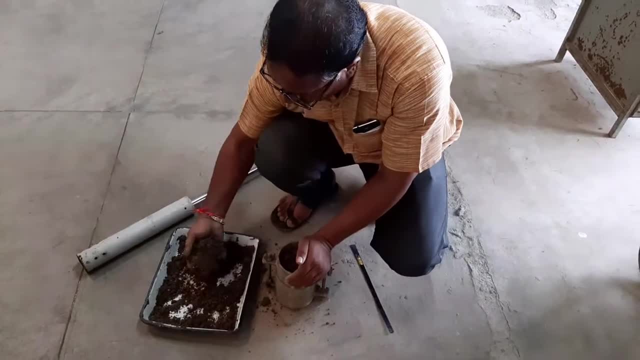 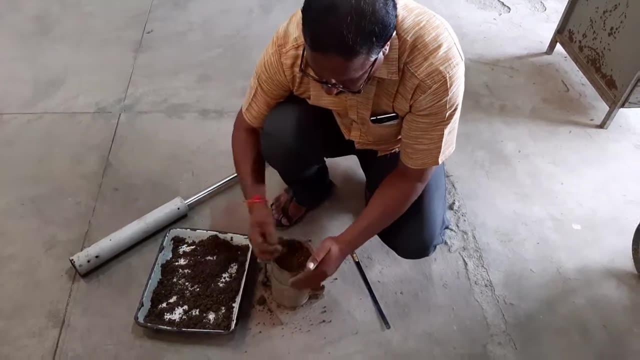 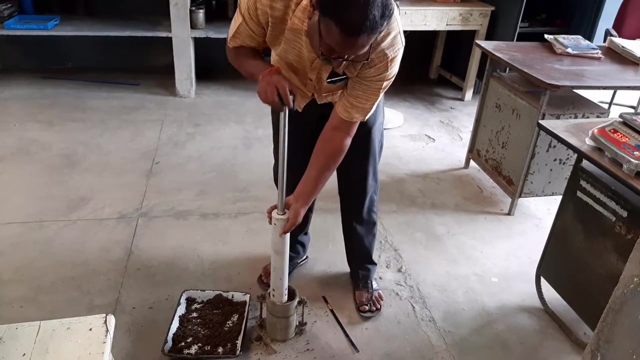 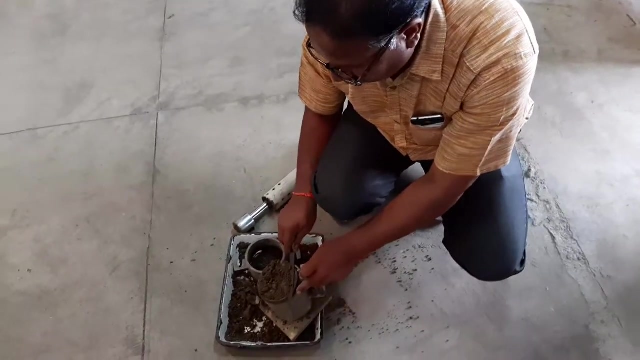 to give 25 number of blows. at the last we will add the third part of our specimen and we will add to the compactor and will again give 25 number of blows by using the steel rammer. after compacting the third part of the soil, at last, we will remove the collar and then we will cut the soil. 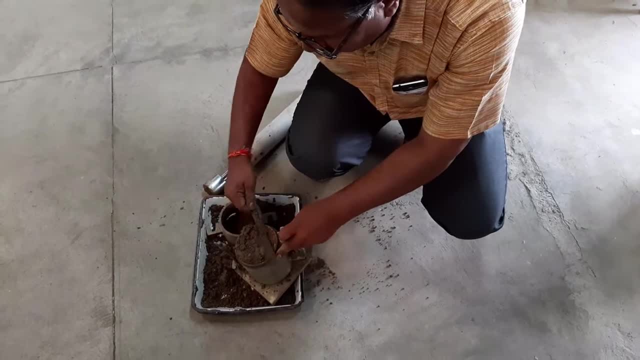 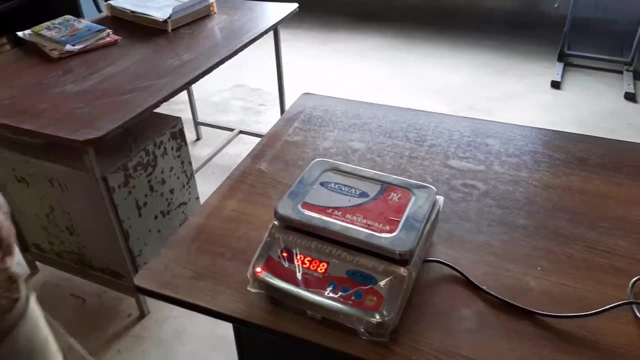 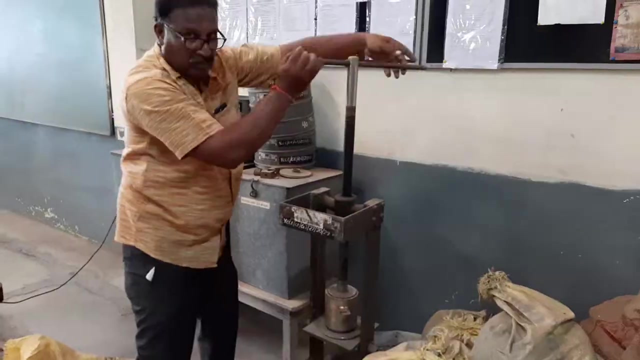 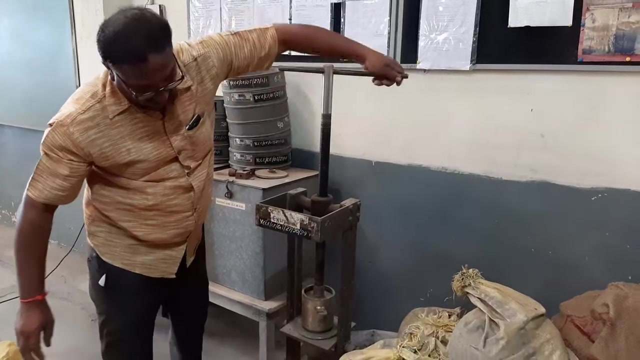 from the top edge of our compactor. we will level it by removing the extra soil from the top of our mold. next process is that we will weight the mold with the soil sample. now for removing the soil we will use the apparatus called as soil excluder. that will remove all the soil from our 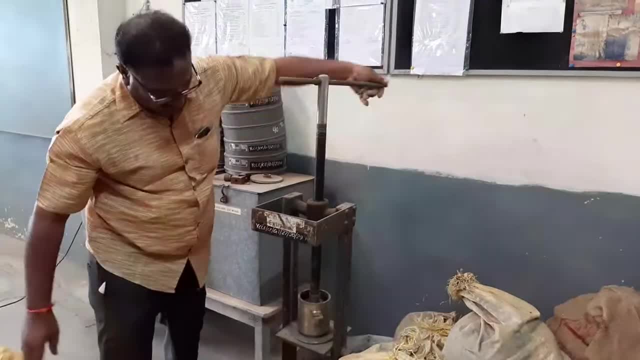 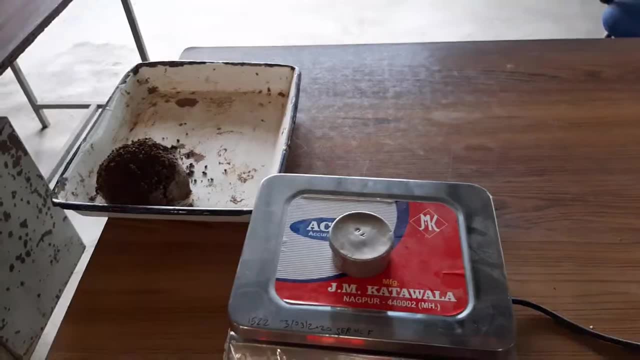 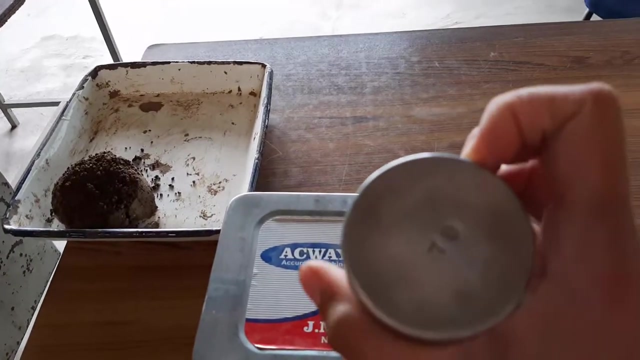 apparatus or the mold similarly, that we have taken into core cutter method. we will collect the soil from the bottom at the bottom plate. now we will determine the moisture content of the soil. for that we need a metal container which is empty, with a metal container number. that is here we are. i am using 78 number of metal container. 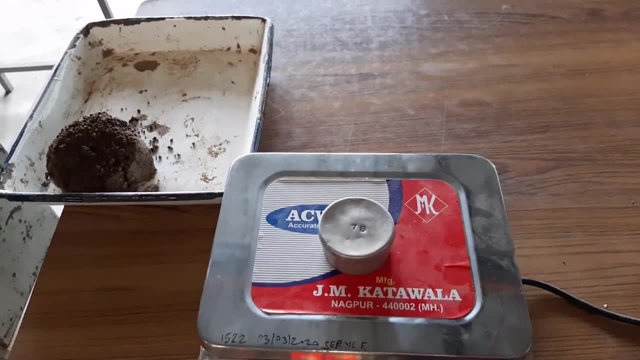 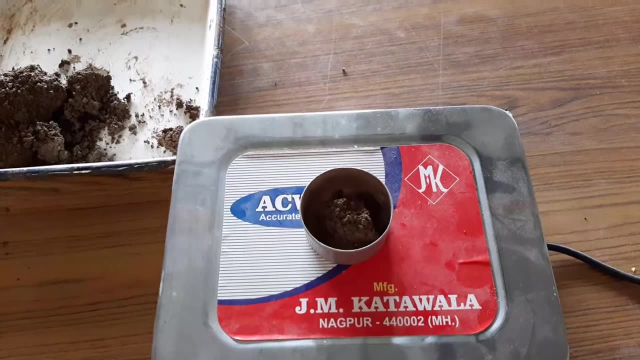 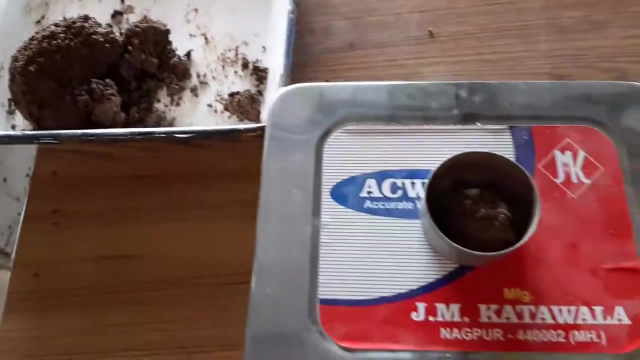 now we will take the empty weight of this metal container. after taking the empty weight of the container, i will put the sample that i have collected from the dense part of our soil which is collected from the mold. i will cover it. i will take the weight of. 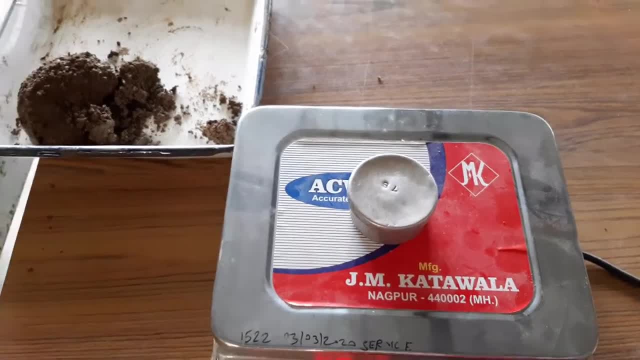 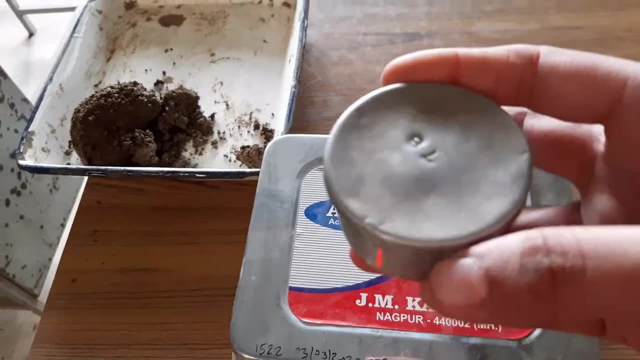 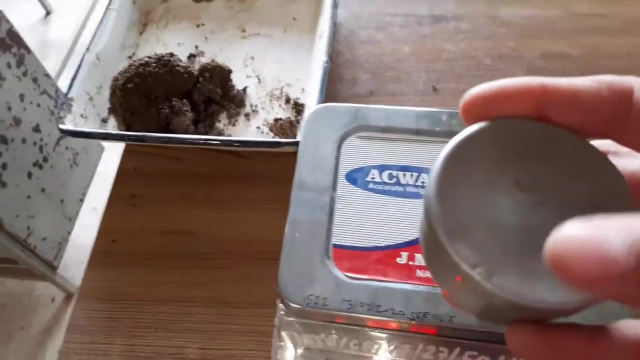 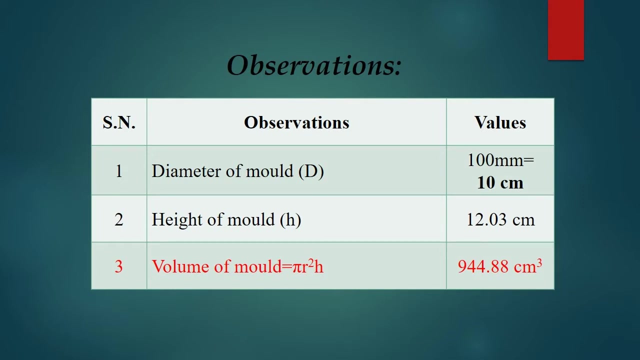 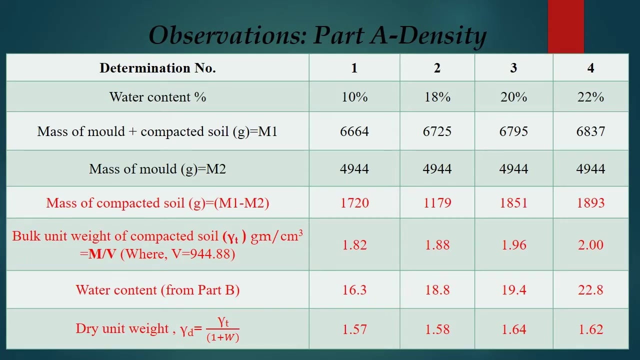 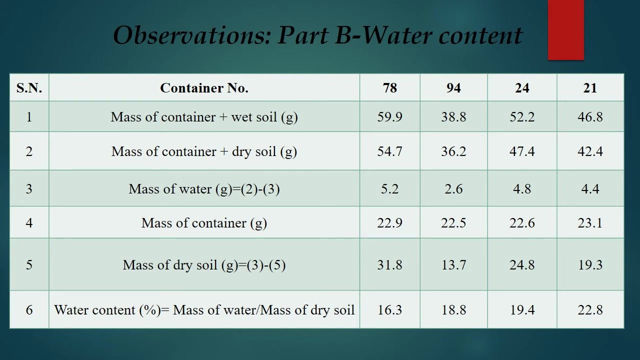 the container with this soil. after this, i will keep the. after this, The metal container is kept in the oven for 24 hours and the reading is noted after 24 hours. The metal container is kept in the oven for 24 hours and the reading is noted after 24 hours. The metal container is kept in the oven for 24 hours and the reading is noted after 24 hours.